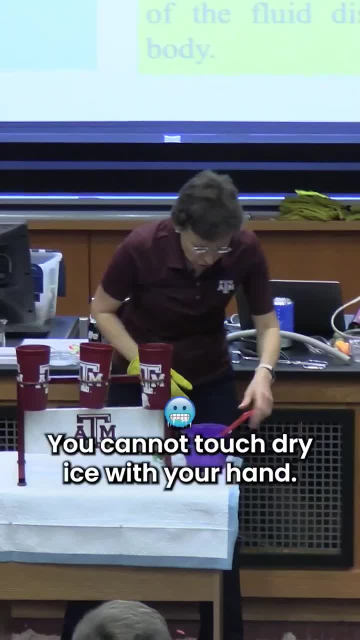 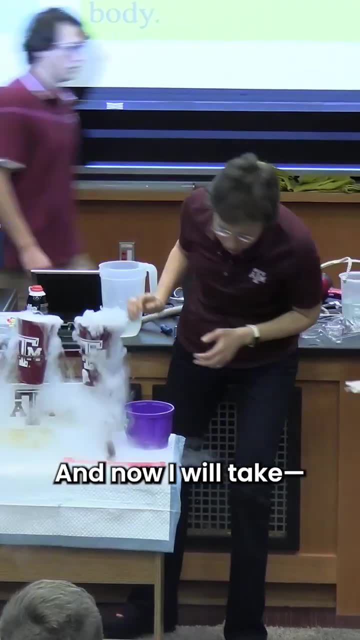 I put a piece of dry ice here. I wear a glove, right, You cannot touch dry ice with your hand. We will add water to increase evaporation. We will add a little bit of water and now I will take- thank you so much, and we will soak this paper towel in bubble solution. Watch. 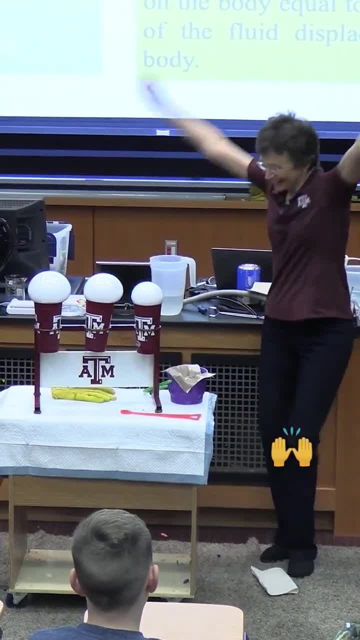 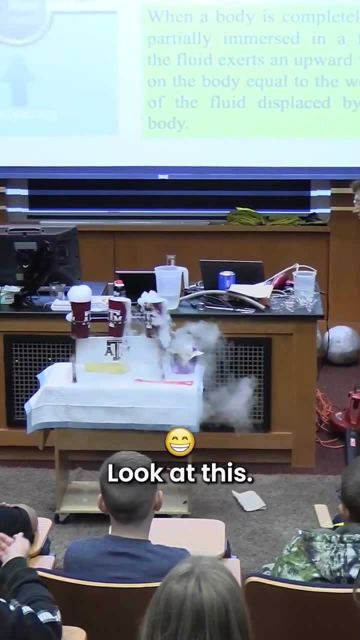 Look at this: We never give up. Look at this.